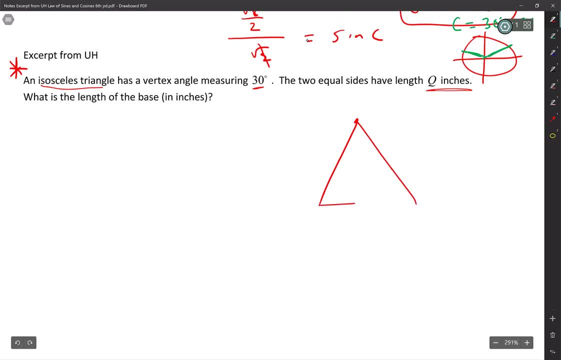 And hopefully you do, guys. An isosceles triangle means that two sides are the same, So I'm going to say those two sides And it's not to scale The vertex angle. that means this is my vertex angle. I'm going to say that's 30 degrees. 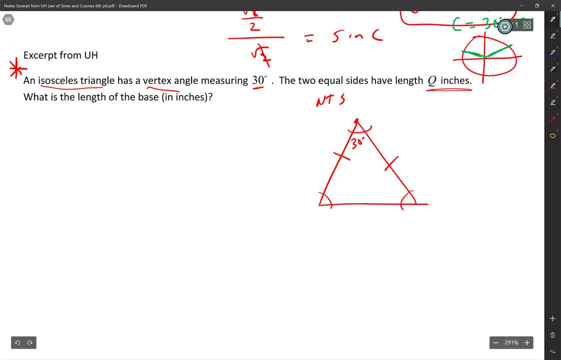 And two equal sides. So these angles here must be congruent. So let's see 180 minus 30. What's that? 150.? And then take the 150 and divide it by two, So these two angles are both. Is that 75?? 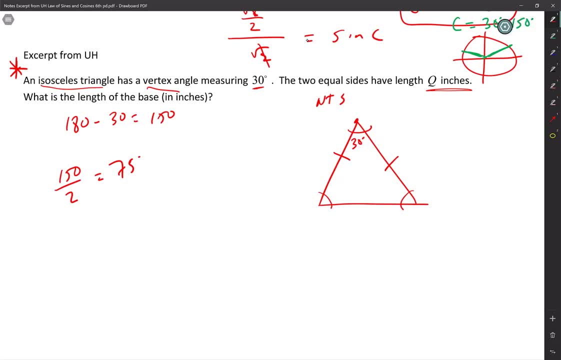 Yeah, 75. I have three quarters and add another three quarters, That's $1.50.. Yep, 75 degrees, 75 degrees, And this is Q, And this is Q. They told me that. What is the length of the base? 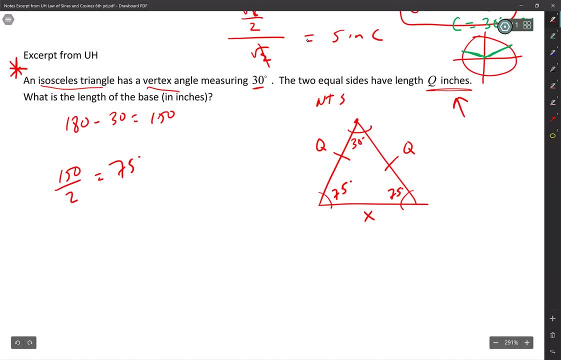 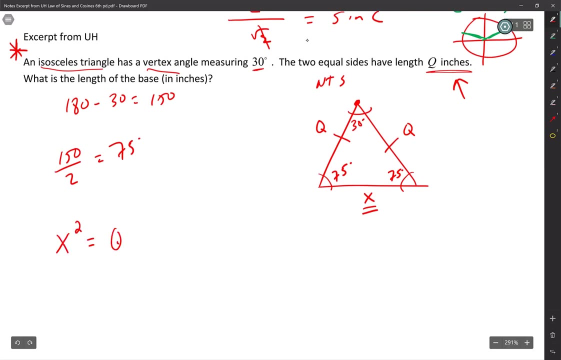 So they want to know the length of that base. I'm going to call it X, So check it out guys. I'm going to use law of cosines. I have the 30 degrees. This is a vertex And I'm trying to figure out what X is. So law of cosines is X squared equals side, So Q squared. 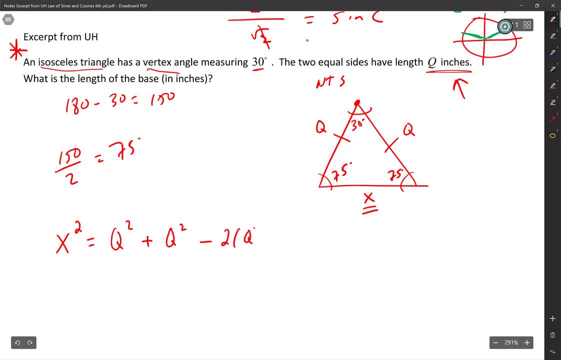 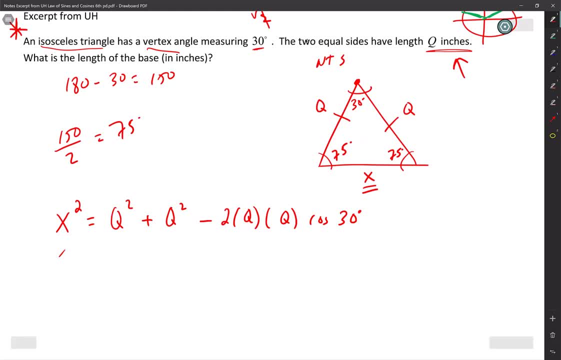 algebra can be kind of hard guys. So here we go: X squared equals. And I got two of these dudes, So I'm going to say 2Q squared minus 2 times Q times Q, That's another 2Q squared, Cosine 30. 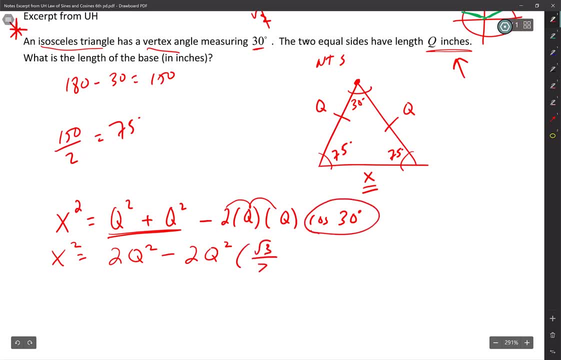 degrees is square root of 3 over 2.. What's up, miss? Yes, I think that's one right, there Is that one? No, Okay, Try You. see back there that laptop. You can take that charger for now See if that one works. 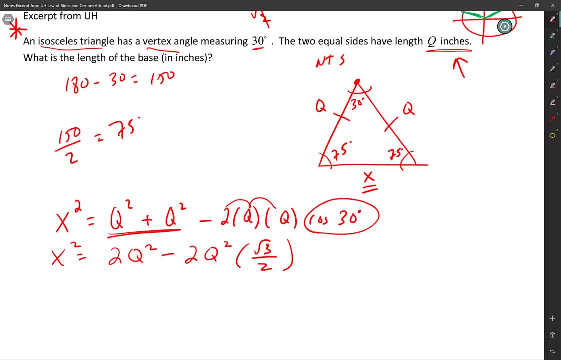 If it doesn't, let me know. No, I do have a charger. Open up that closet there and then look in the bottom And then way in the bottom See if there's any wires, or maybe in the middle of it. I'm sorry.